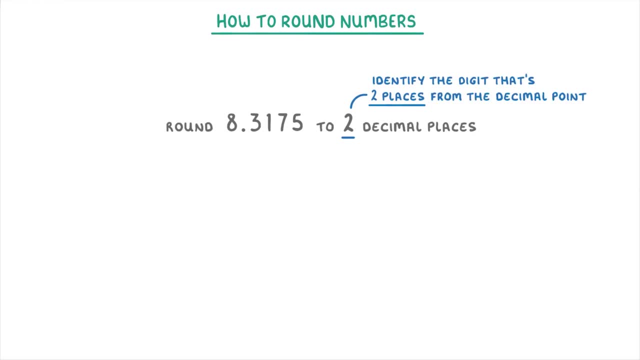 the digit, that's two places from the decimal point, which in this case is the 1.. We call this one the last digit because it's the last digit that we want to have in our answer, The digit to the immediate right of this. so the 7, is called the decider because this: 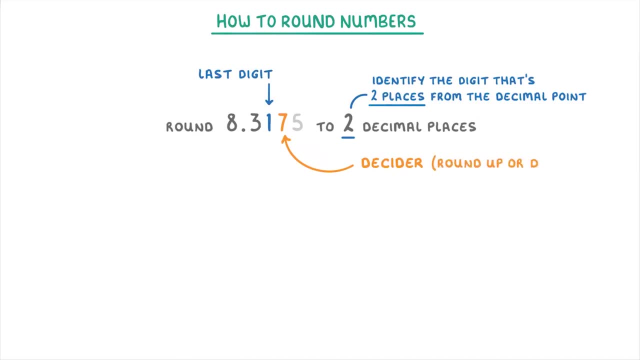 is the one that we look at to decide whether we need to round up or round down. If the last digit is one, two, three or four, then we leave the last digit as it is. But if it's five or higher- so five, six, seven, eight or nine- then we round up the last digit. 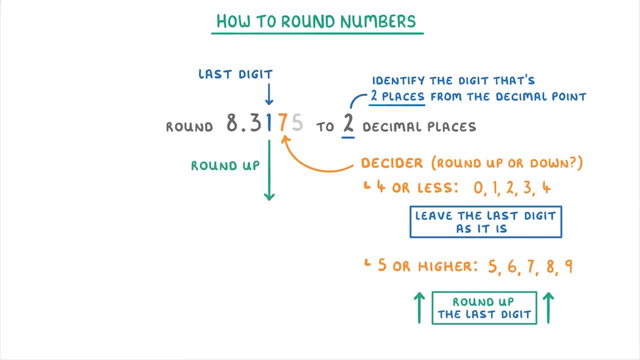 So, as our decider is seven, we have to round our last digit up and change the one to a two, And then, to finish, we just remove all of these other digits that come after the last digit rounded: 8.3175 to 8.32.. 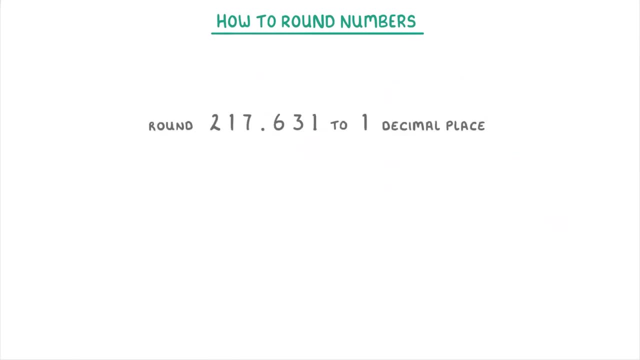 In this next one we're being asked to round 217.631 to one decimal place. So, because we're rounding to one decimal place, our last digit will be this: 6, because that's one place to the right of the decimal points. 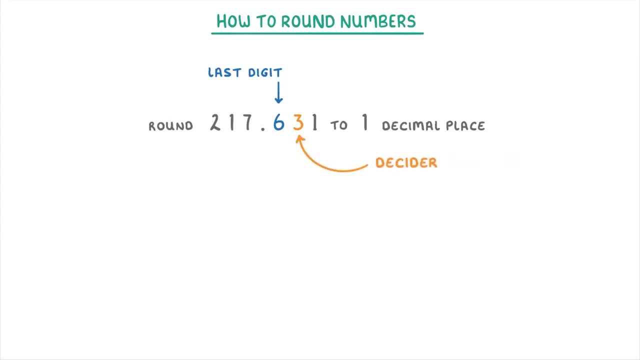 And so the 3 will be the decider, Because 3 is in the 4 or less group. it tells us that we're going to have to round down And remember, when we round down, we keep the last digit as it is. 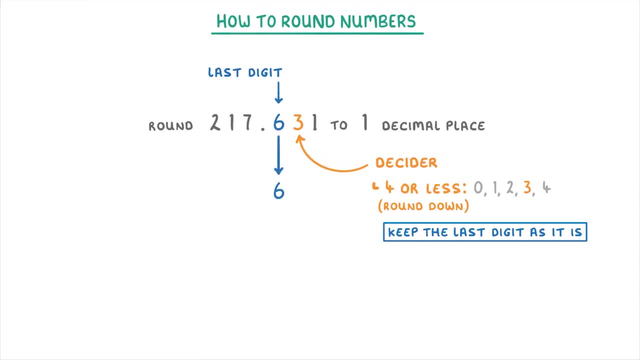 So the 6 stays as a 6.. This means that all we have to do is rewrite it as 217.6.. And that's it So effectively. we just got rid of the 3 in the last digit, And now we've got 217.631.. 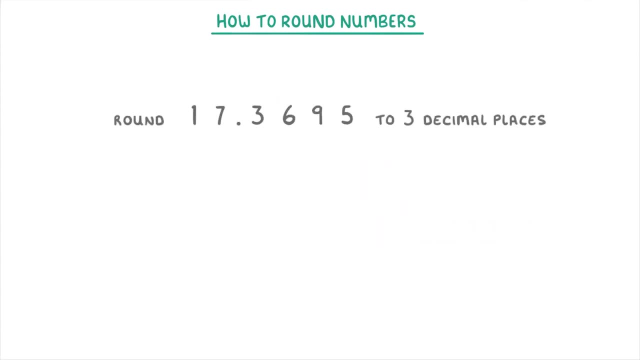 In this last question we're rounding 17.3695 to three decimal places. So this time the 9 would be our last digit, because it's three places to the right of the decimal point, And the decider would be the 5, because that's the next digit to the right. 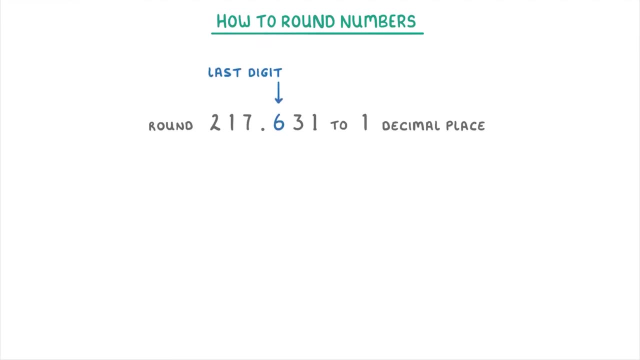 So, because we're rounding to one decimal place, our last digit will be this: 6, because that's one place to the right of the decimal points, And so the 3 will be the decider, Because 3 is in the 4 or less group. it tells us that we're going to have to round down. 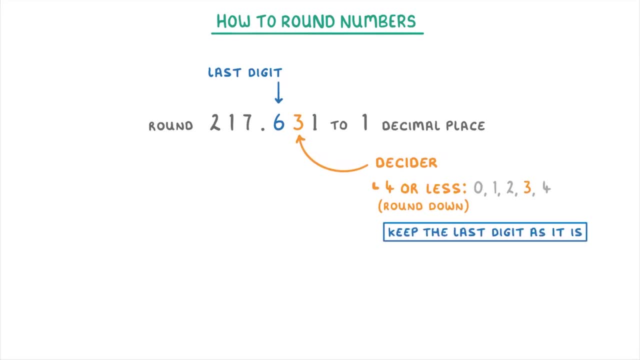 And remember, when we round down, we keep the last digit as it is, So the 6 stays as a 6.. This means that all we have to do is rewrite it as 217.6.. And that's it So effectively. we just got rid of the 3 in the last digit. 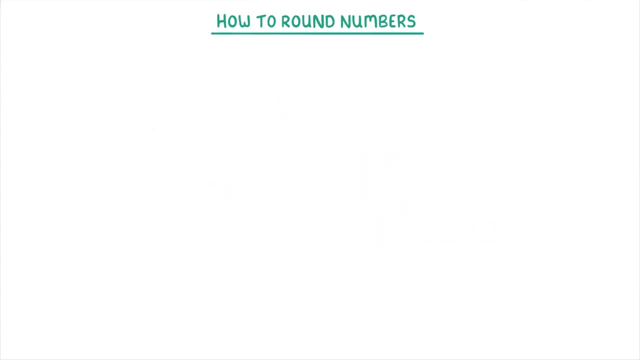 And now we've got 217.631.. In this last question we're rounding 17.3695 to three decimal places. So this time the 9 would be our last digit because it's three places to the right of the decimal point. 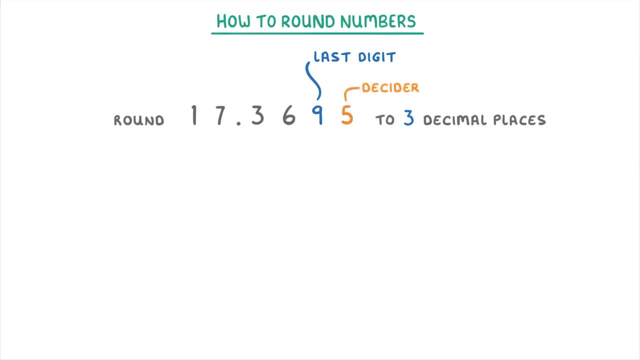 And the decider would be the 5, because that's the next digit to the right, Because the decider is a 5,. it means we're going to have to round our last digit to the right of the decimal point. So we're going to have to round our last digit to the right of the decimal point. 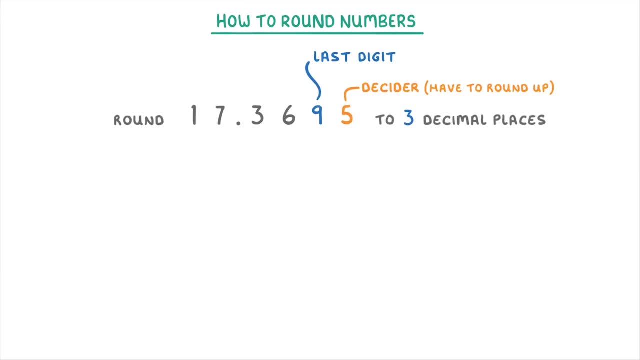 So we're going to have to round our last digit up. But when you have to round up a 9, it is kind of tricky, because the 9 gets rounded up to a 10, which means that the 1 is in the column to the left. 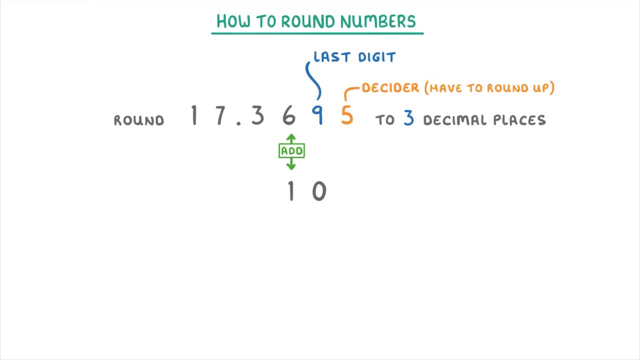 And so we have to add it to the 6.. So in this case, our 6 becomes a 7., And we bring down the 0 as well, so that overall we end up with 17.370.. Another way of thinking about it that you might find interesting is to think about the. 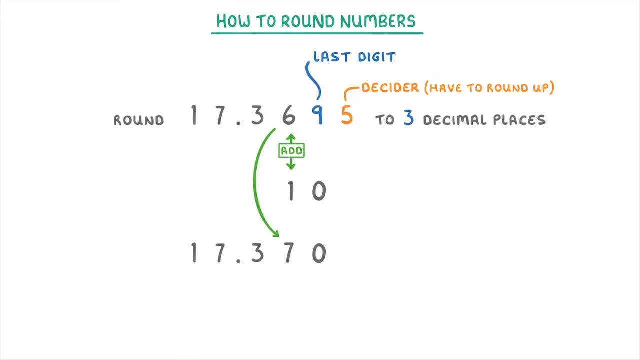 number of digits, And this is kind of easy, It's to think of it as if we're rounding this 69 up to 70.. The last thing to point out is that we have to keep this 0 in our answer Because, remember, we were asked to round three decimal places. 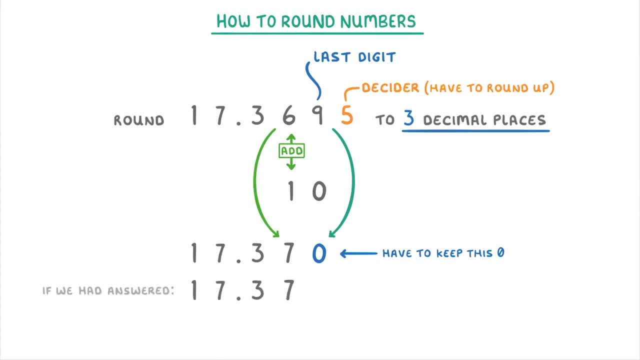 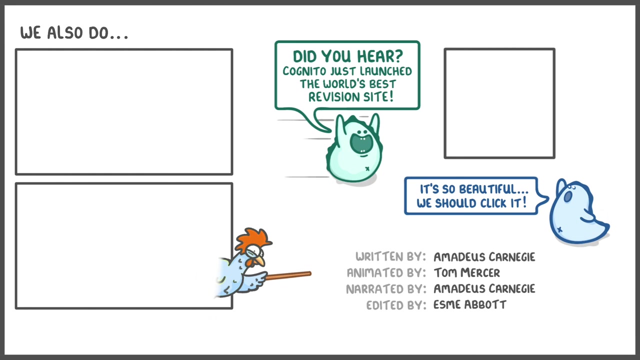 So if you just wrote 17.37 instead, then you wouldn't get all the marks, because that answer only has two decimal places. Anyway, that's everything for this video, So I hope that made sense. If it was useful, then please do like and subscribe.